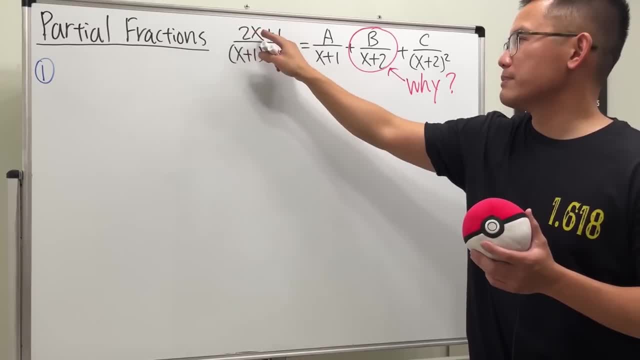 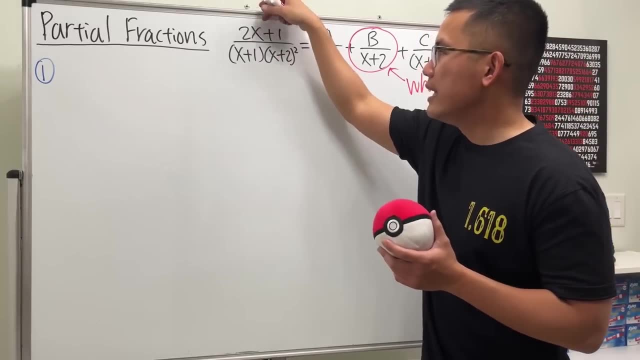 This could have been 3x-11 or 2x-217.. The setup would still be the same, as long as the degree is strictly less than the degree on the bottom. The degree here is 1, the degree here is 1 plus 2,, which is 3.. 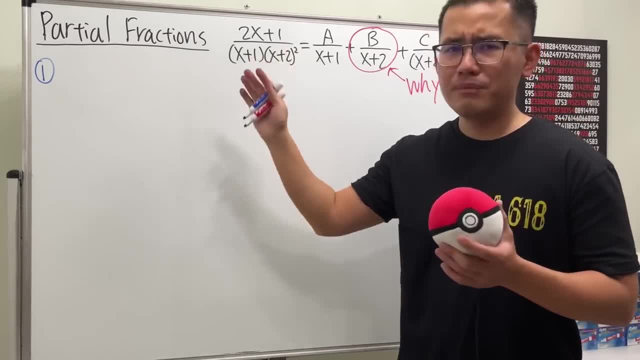 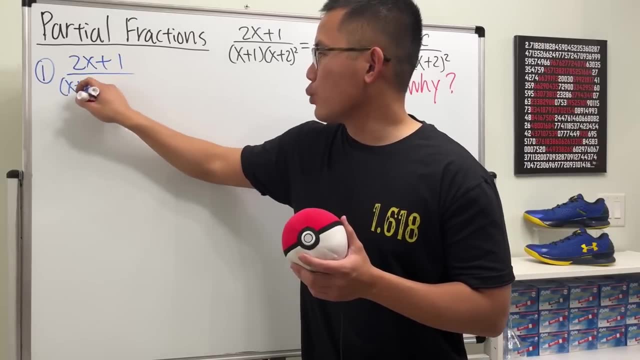 So the setup would be like this And let's just use the same numerator, 2x plus 1.. So if we take a look at 2x plus 1 over, if we just have x plus 1 times x plus 2.. 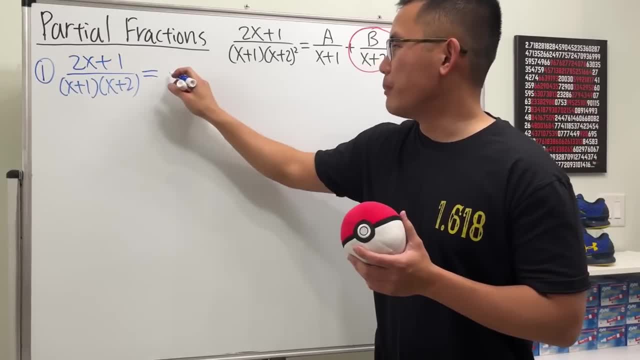 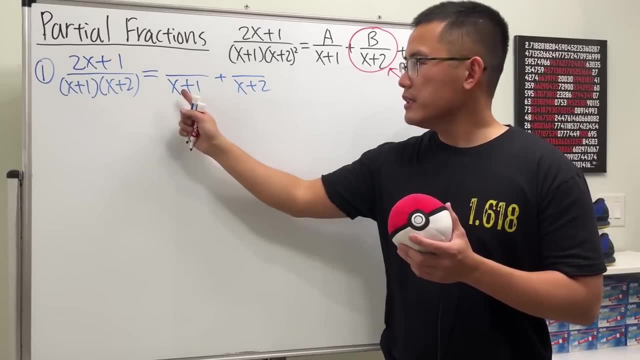 This is nice. This is everybody's favorite, because we can just break them apart with x plus 1 right here, and then the second fraction, we get x plus 2.. Notice that they are just both linear, meaning degree 1, so the top will be just constants. 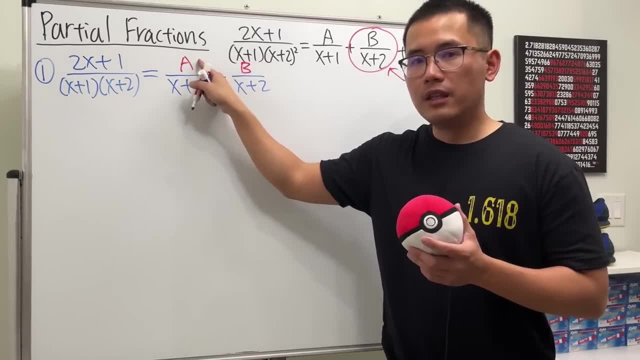 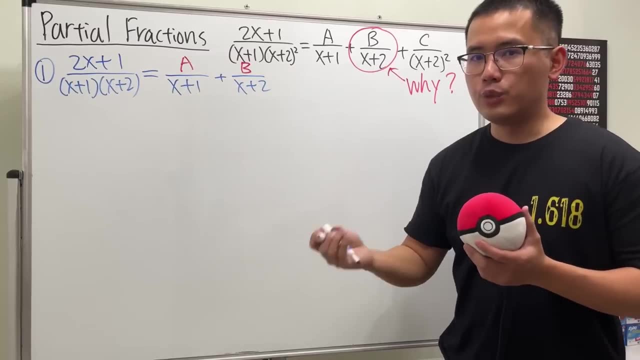 Because you always want to make sure when you set up the degree on the top is 1 less than the degree on the bottom. So degree here is 1, that means the top right here is degree 0,, meaning just constants. 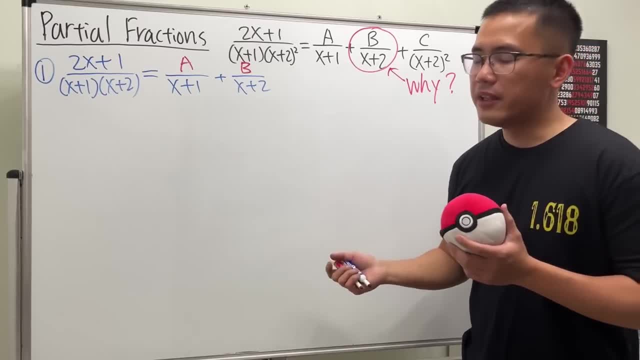 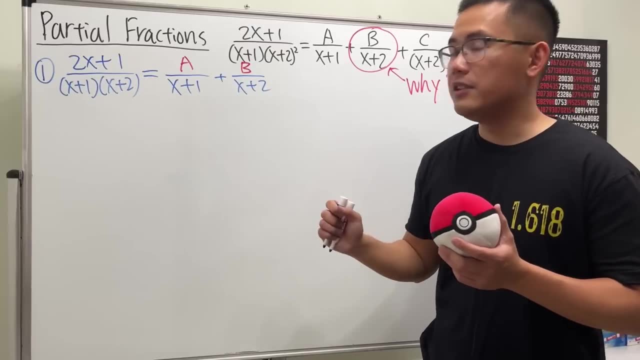 And then we can talk about. We'll talk about how to get the a and b by using the Kavra method in another video, but this is the setup first, when we have two different factors and they are both linear. Now let's take a look at the second one. 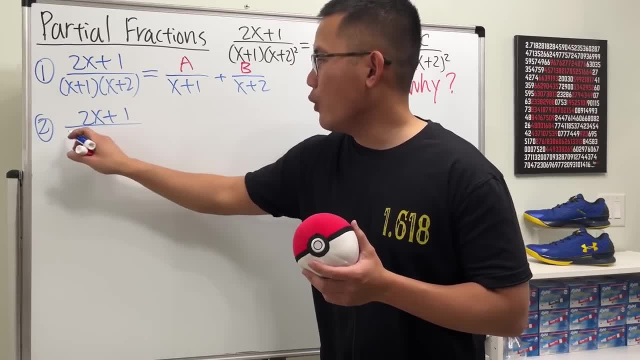 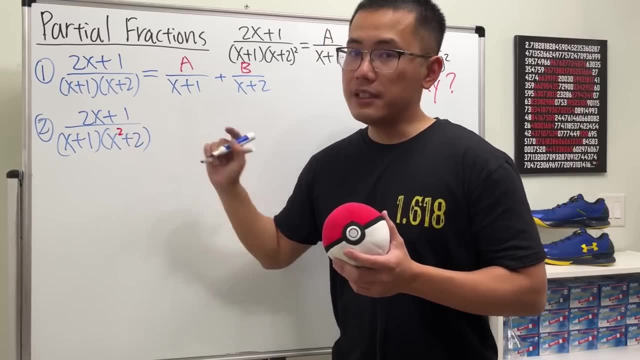 What if we have a quadratic? let's say 2x plus 1 on the top over x plus 1, but this is x squared plus 2.. This right here is a quadratic. It's kind of similar to this because technically this is also quadratic, but the thing is that 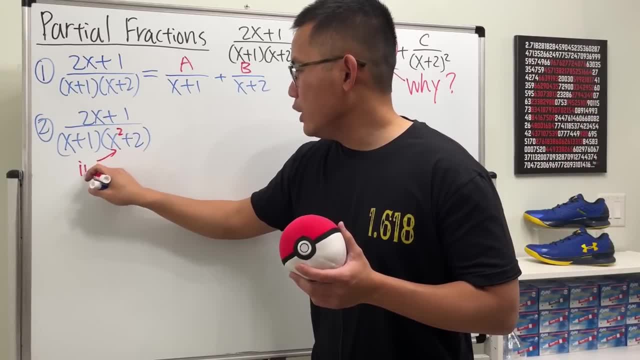 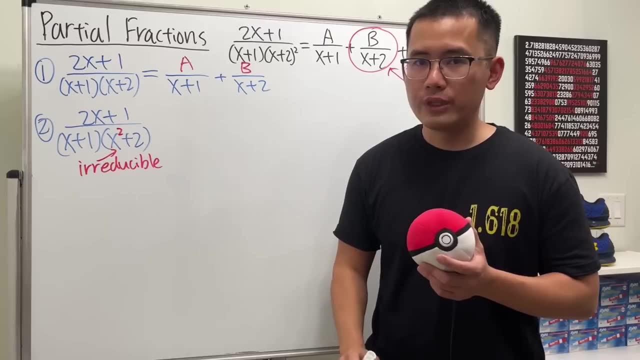 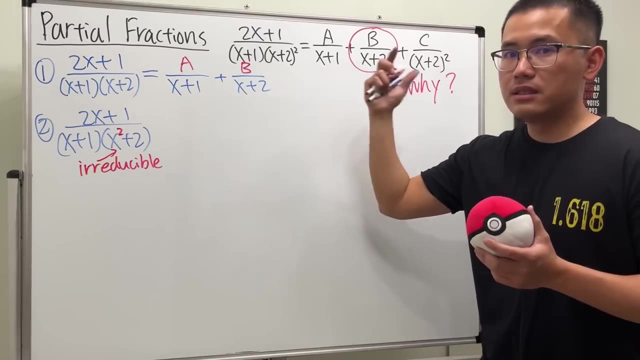 this right here is actually an irreducible quadratic, meaning that we cannot factor this anymore with real numbers, So we just have to deal with this right here. But technically, this right here is what Means: x plus 2 times x plus 2.. 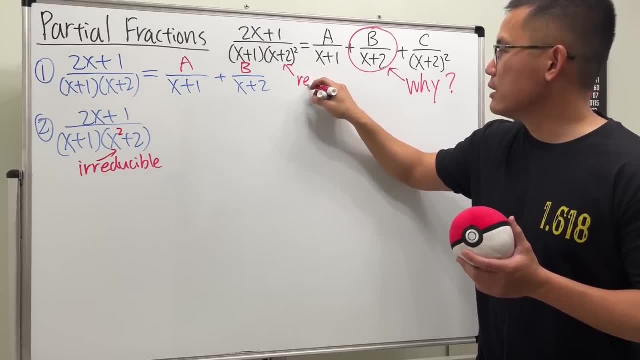 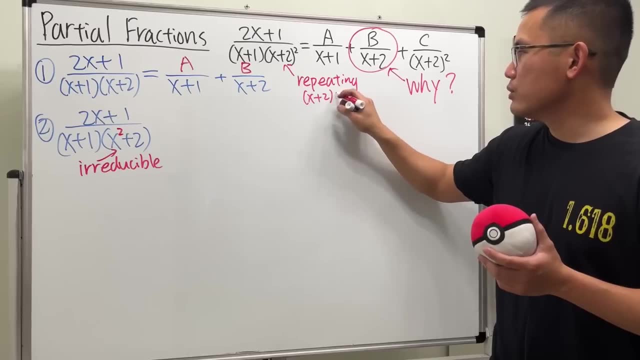 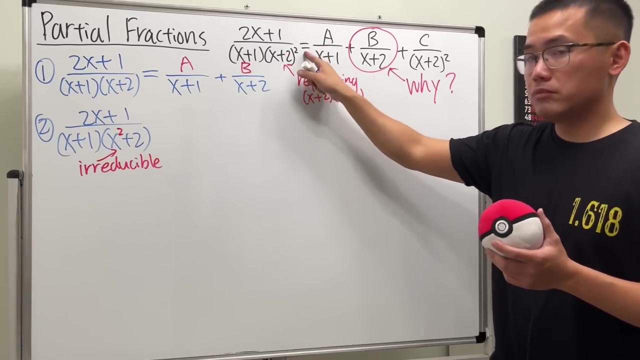 This right here is a repeating factor. so I'll just say this is a repeating factor and this right here We can look at it as x plus 2 times x plus 2.. So when you have a repeating factor like this, you have a power on the outside of the parentheses. 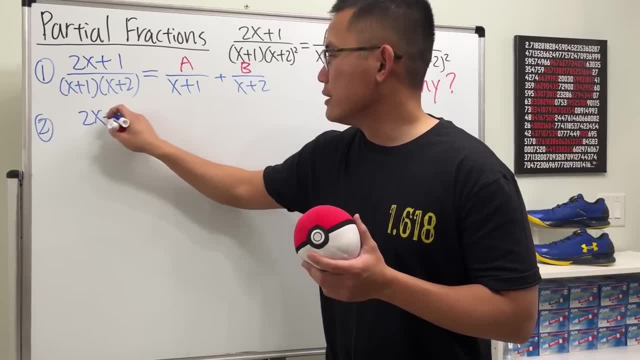 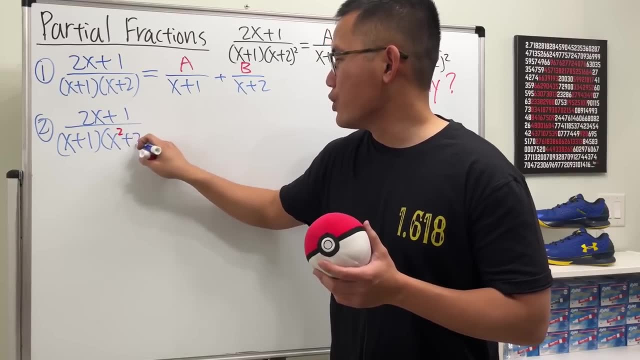 Now let's take a look at the second one. What if we have a quadratic, let's say 2x plus 1 on the top, over x plus 1, but this is x squared plus 2. 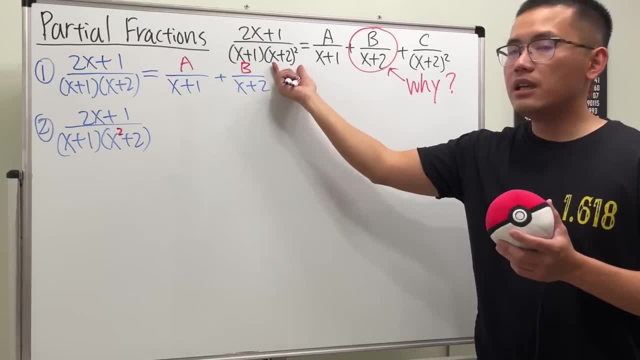 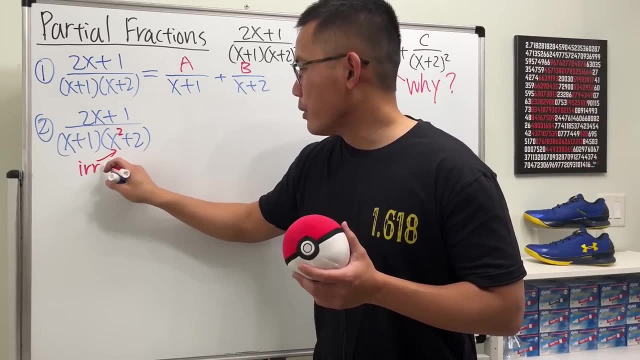 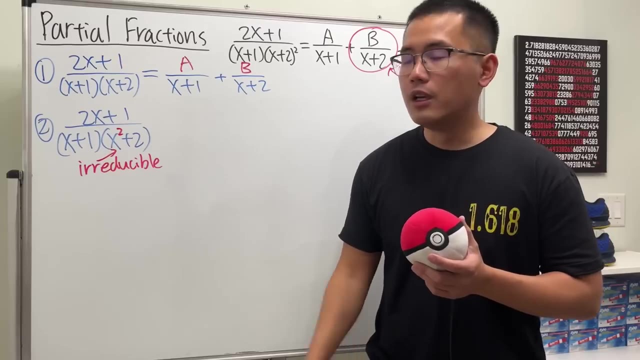 This right here is a quadratic. It's kind of similar to this, because technically, this is also quadratic, but the thing is that, this right here is actually an irreducible quadratic, meaning that we cannot factor this anymore with real numbers, so we just have to deal with this right here. 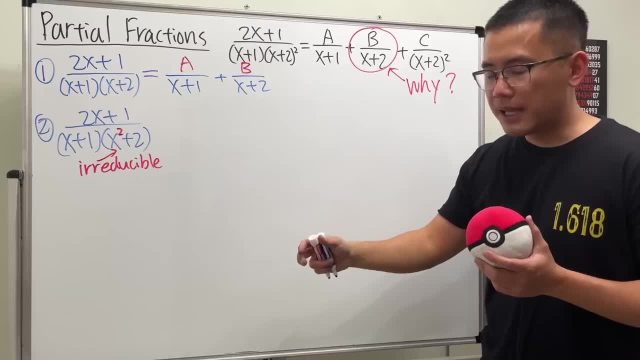 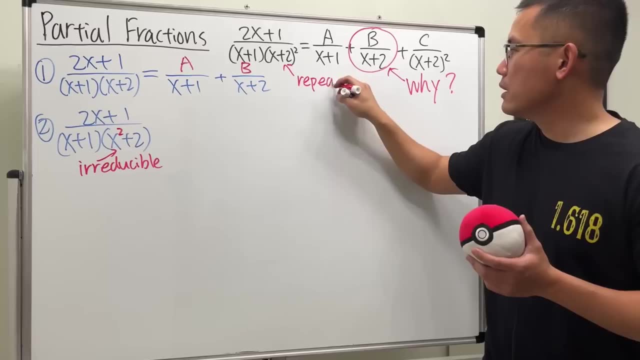 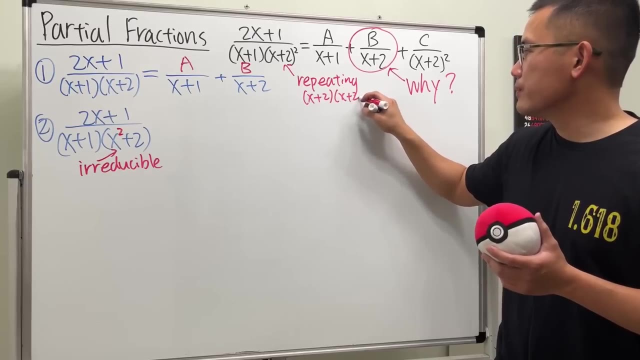 But technically, this right here is what? Means x plus 2 times x plus 2. This right here is a repeating factor, so I'll just say, this is a repeating factor, and this right here. We can look at it as x plus 2 times x plus 2. 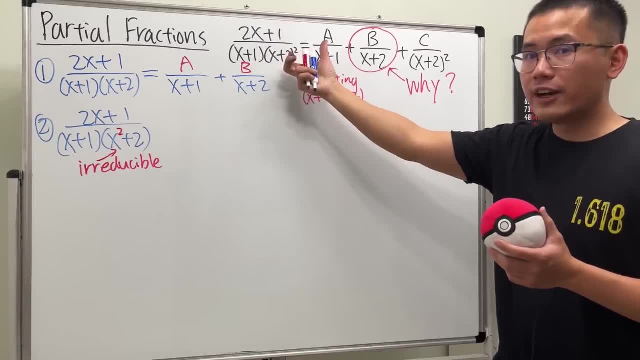 So when you have a repeating factor like this, you have a power on the outside of the parentheses, and then you will have to do things like that. But let's talk about that later. 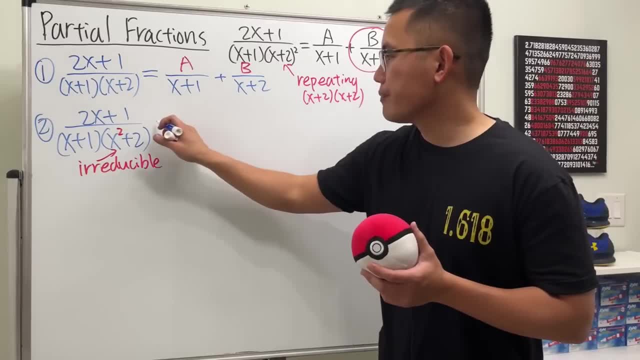 How do we take care of an irreducible quadratic? Have a look. 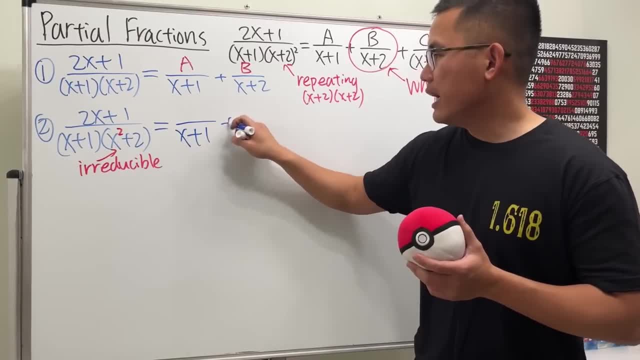 Again, the first fraction will have x plus 1 on the bottom, and then for the second fraction, we'll just use this. 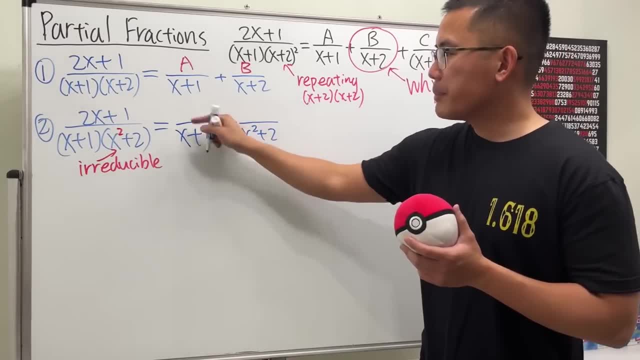 That's x squared plus 2. On the top here, it will just be a constant. 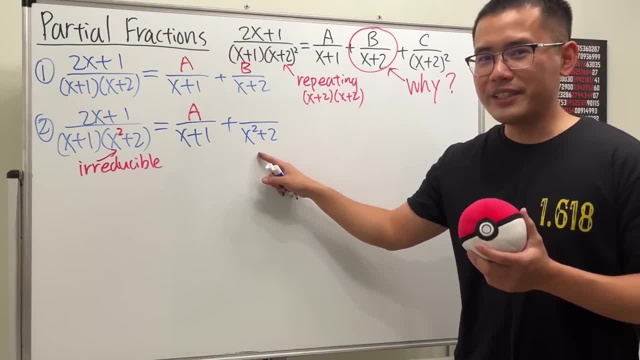 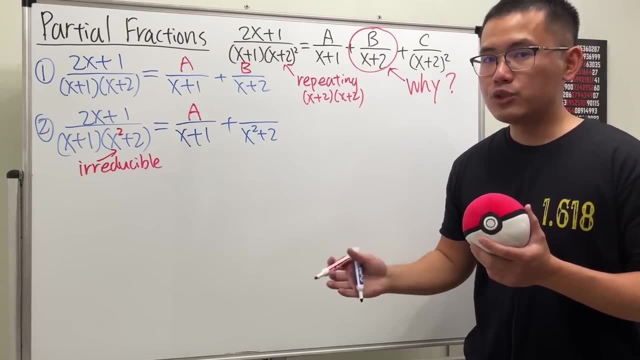 But for this right here. Because it's a quadratic on the bottom, and the top has to be one degree less than the bottom, so we will have to set up a linear, and you have to make sure you put down the general form, so we get bx plus c. Done. 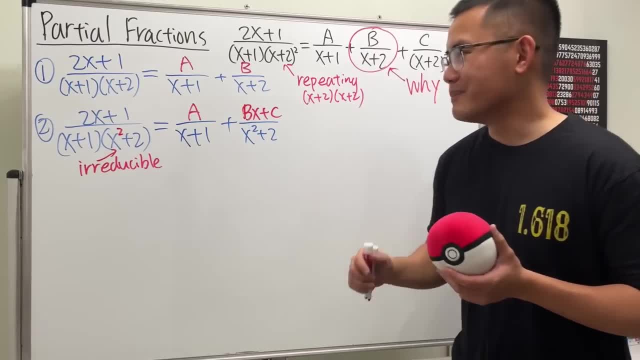 And of course, to solve for a, b, c, it's going to take some time, but maybe another video. All right. Number three. 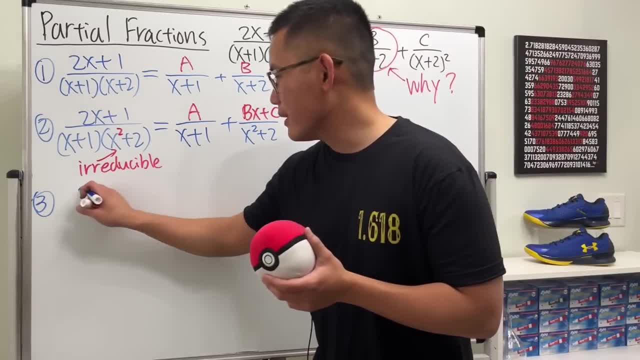 Check this out. I will still give you a quadratic, but this one. Let's say we have 2x plus 1. Over. 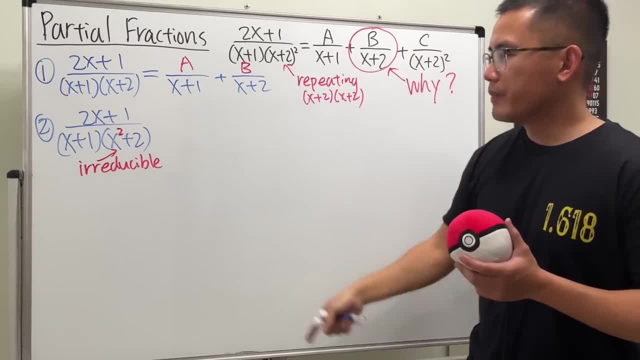 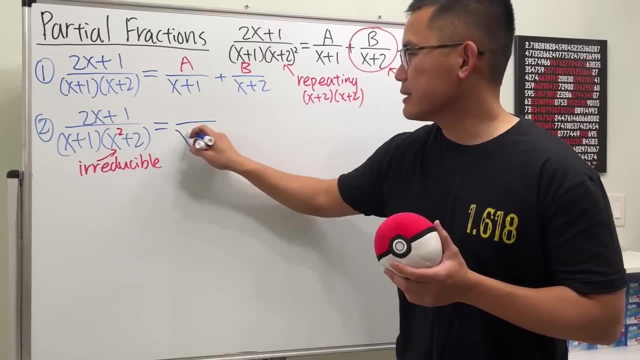 and then you will have to do things like that, But let's talk about that later. How do we take care of an irreducible quadratic? Have a look Again. the first fraction will have x plus 1 on the bottom, and then for the second fraction, 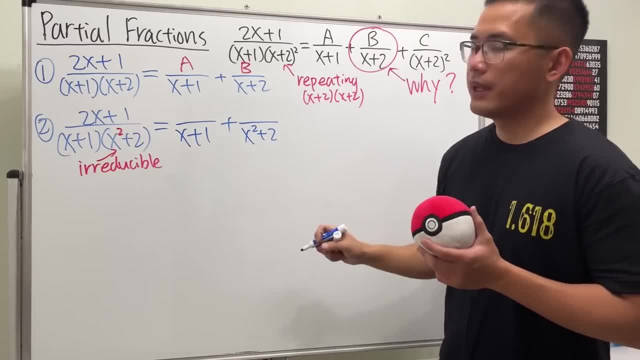 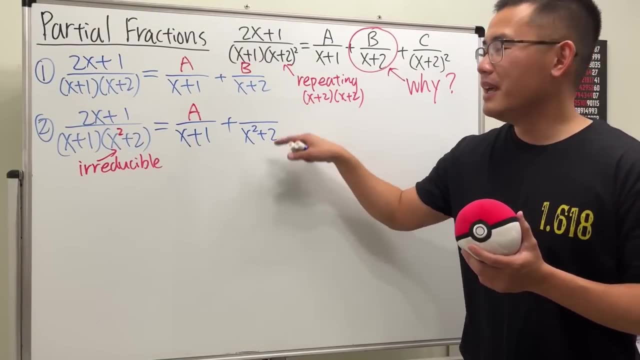 we'll just use this. That's x squared plus 2.. On the top, here it will just be a constant. But for this right here, Because it's a quadratic on the bottom and the top has to be 1 degree less than the bottom. 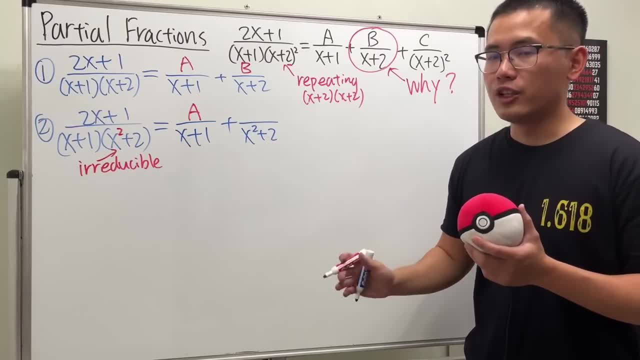 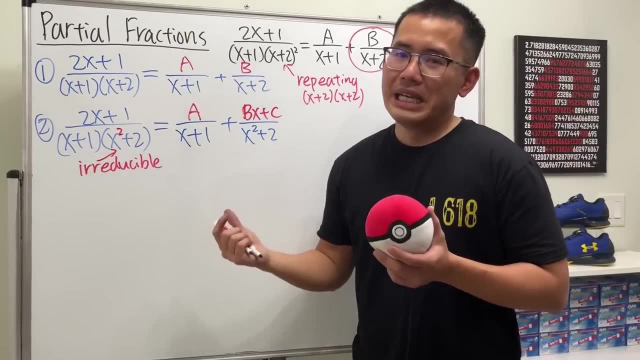 so we will have to set up a linear and you have to make sure you put on the general form so we get bx plus c Done And of course, to solve for a, b, c. it's going to take some time, but maybe another. 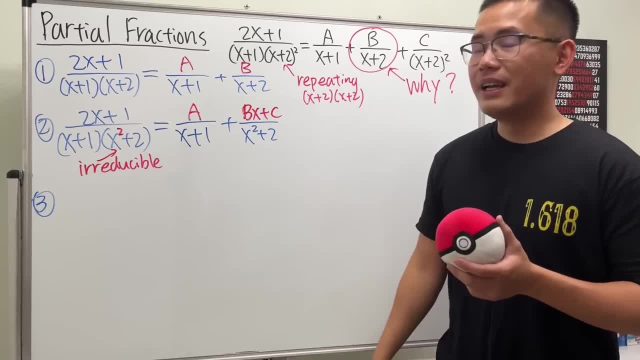 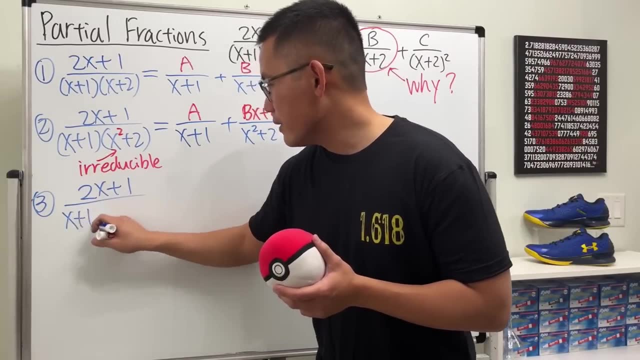 video. All right, Number three: Check this out. I will still give you a quadratic, But this one. Let's say we have 2x plus 1.. Over x plus 1 here And here I will just multiply it with x squared. 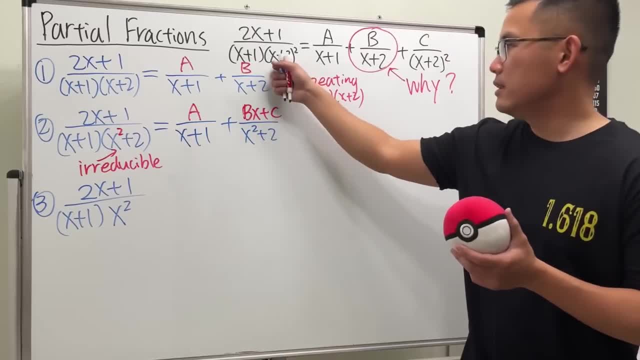 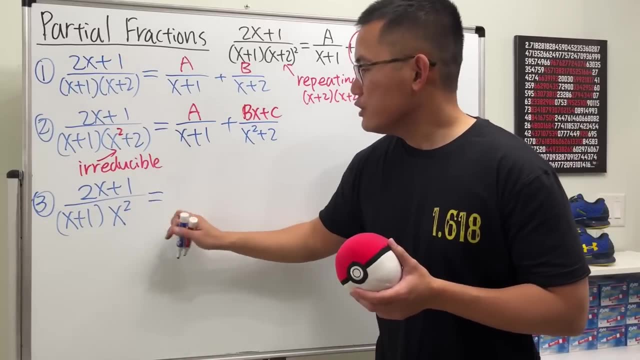 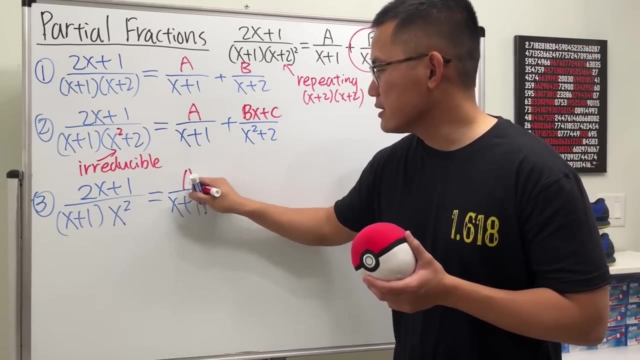 This is also quadratic, But this quadratic is similar than this, Because this right here means what x times x? All right, Okay, Let's use the same strategy than how we set this up earlier. I'm going to first write down the x plus 1 here, which is just a constant on the top. 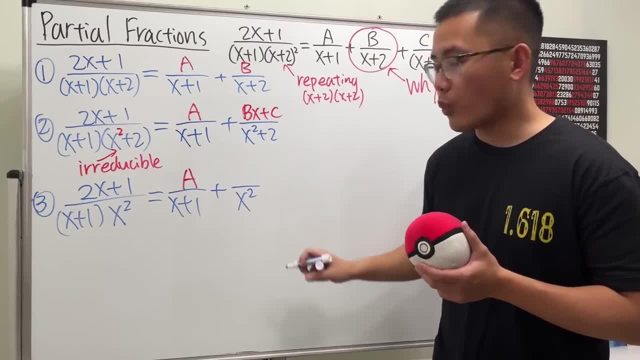 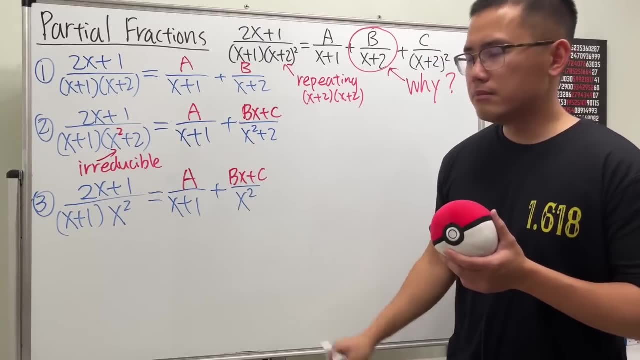 But for this one, okay, I will just keep it as how it is, which is x squared, But at the top we'll just write down the x plus 1 here, which is just a constant on the top, But at the top we'll be a linear meaning: bx plus c. 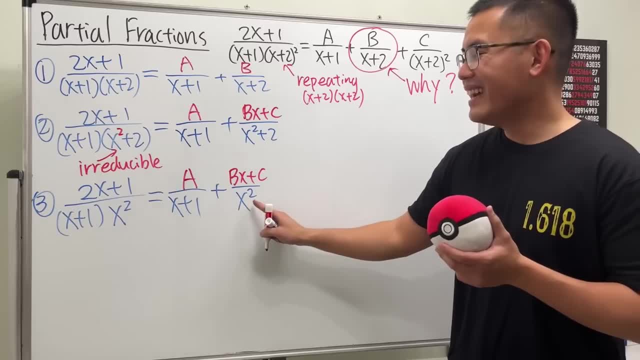 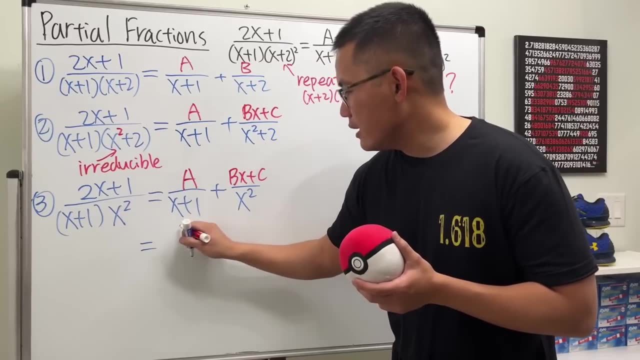 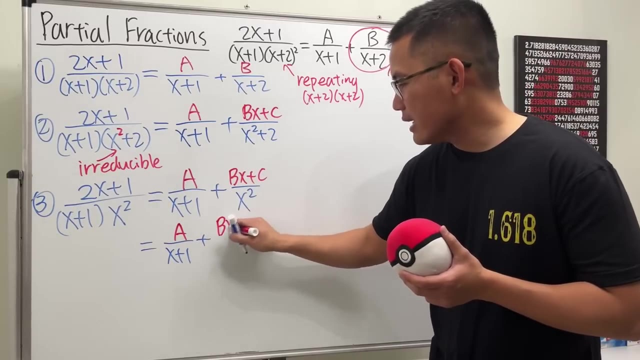 But do we recognize what we can do with this part? See, the bottom here has just one term, so that we can actually just split the fraction and we will get, okay, still a over x plus 1.. But for the second part we can just write this as bx over x squared first and then. 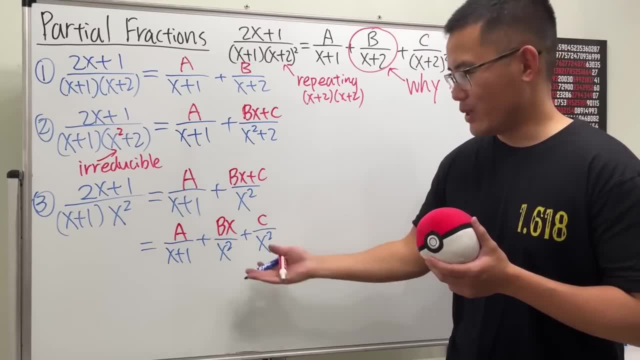 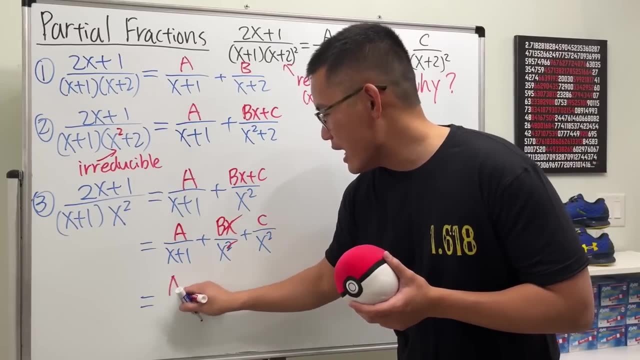 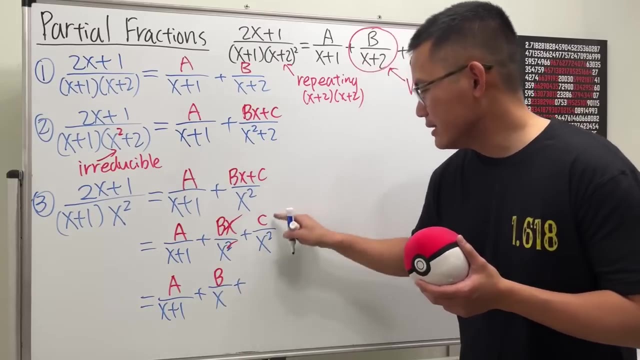 c over x squared. Okay, And what can we do right here? Yes, We can cancel, cancel. So, ladies and gentlemen, we will end up with a over x plus 1, and then plus b over x, and then plus c over x squared. 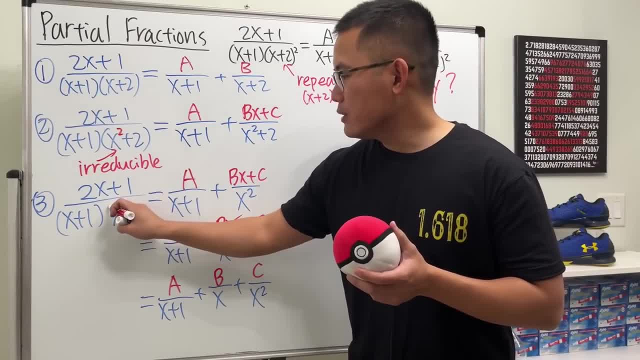 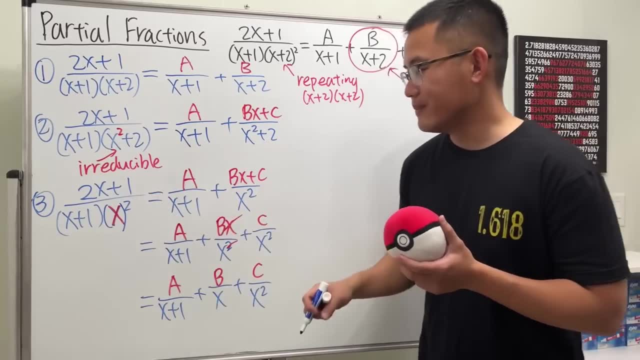 As you can see, right here, we have x squared- and please look at this- x squared as x times x, so we can put the square on our side. It's a repeating factor, But when we set this up, yes, we will have the x squared here, but we also need x to 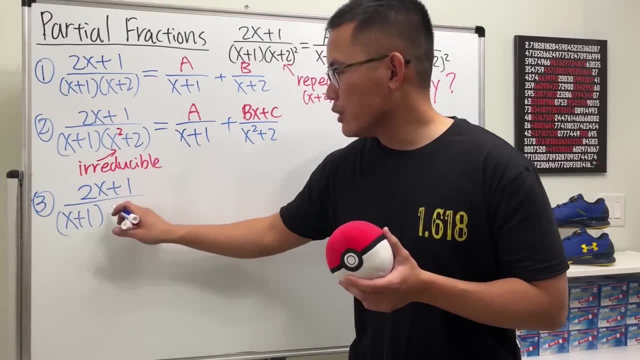 X plus 1 here. And here, I will just multiply it with x squared. This is also quadratic. 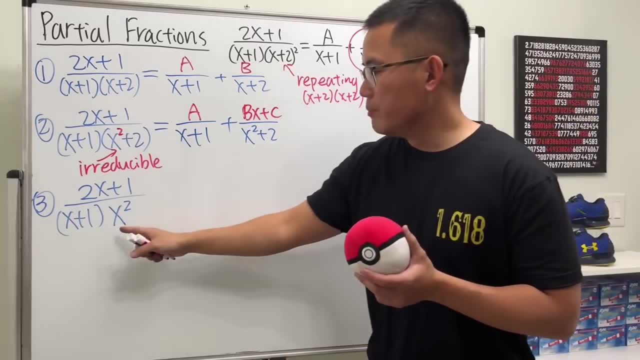 But this quadratic is similar than this. Because this right here means what? X times x. All right? Okay. 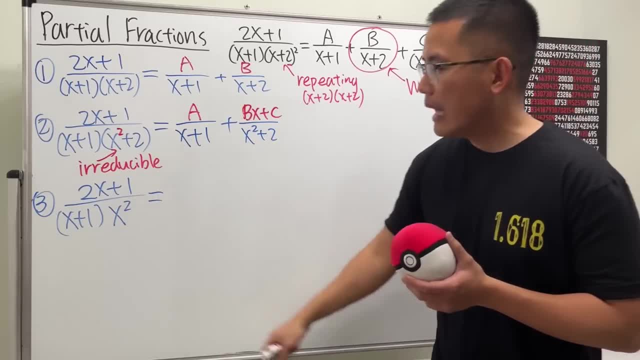 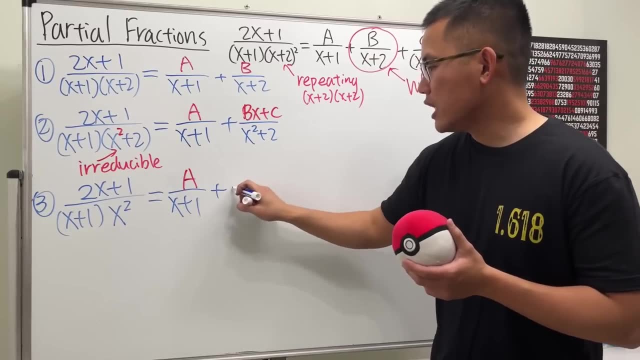 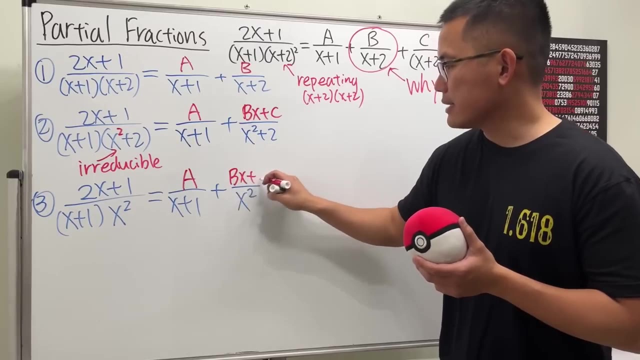 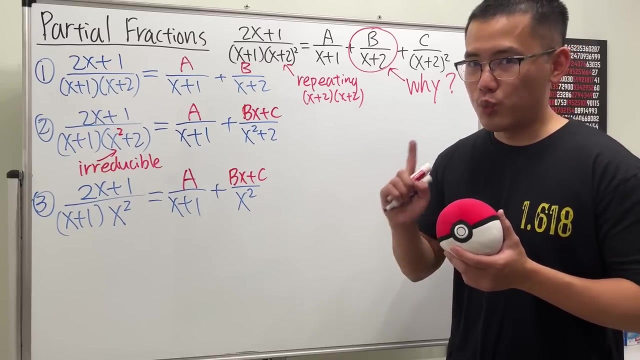 Let's use the same strategy that how we set this up earlier. I'm going to first write down the x plus 1 here, which is just a constant on the top. But for this one, okay, I will just keep it as how it is, which is x squared. But. The top will be a linear, meaning bx plus c. But do we recognize what we can do with this part? See? The bottom here has just one term. 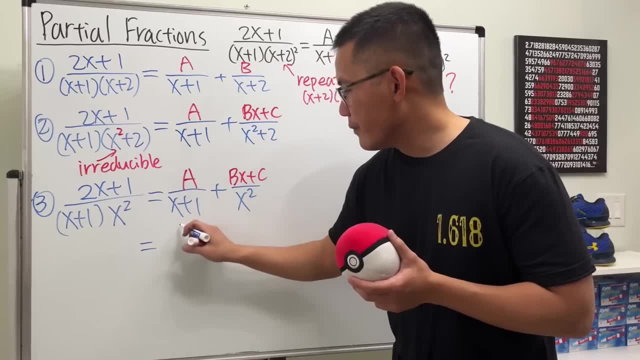 So that we can actually just split the fraction, and we will get, okay, still a over x plus 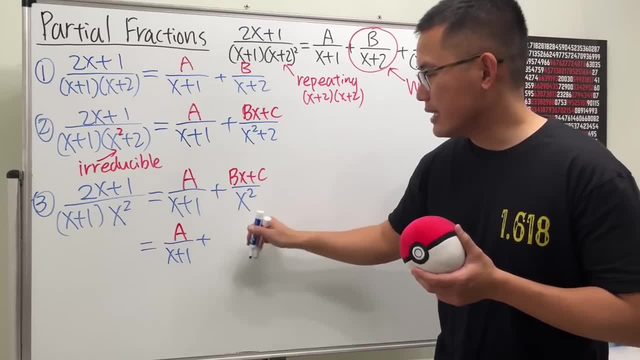 1. But for the second part, we can just write this as bx over x squared first, and then c over x squared. 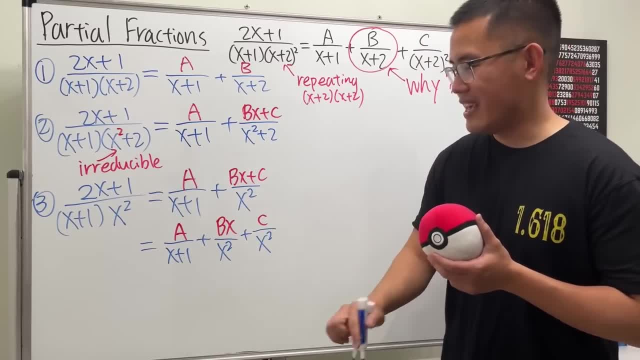 And what can we do? Right? What can we do right here? Yes. We can cancel. Cancel. 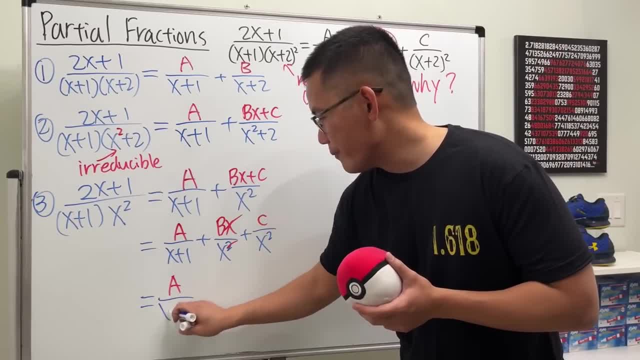 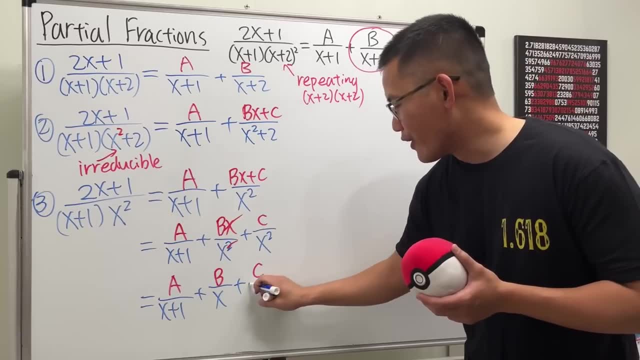 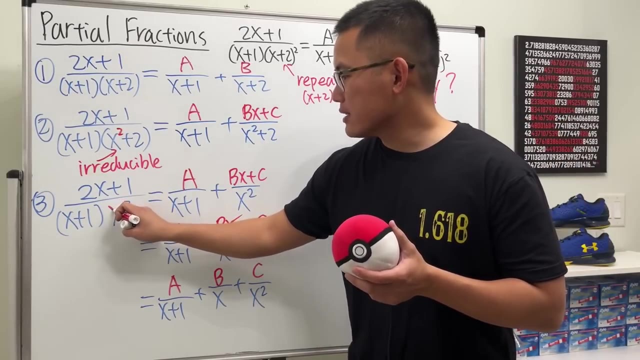 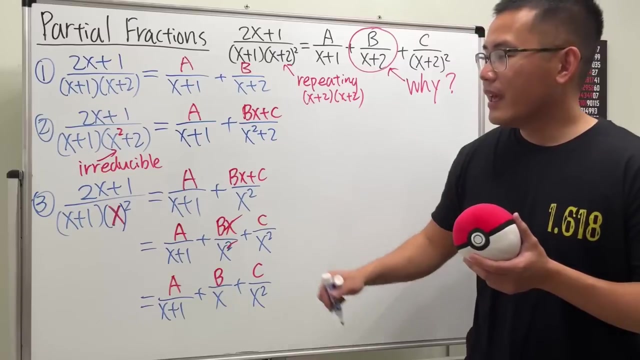 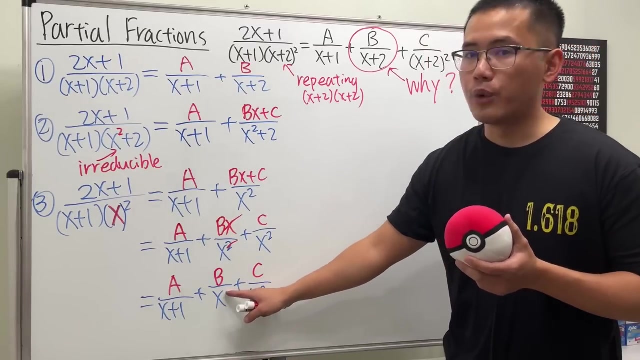 So, ladies and gentlemen, we will end up with a over x plus 1, and then plus b over x, and then plus c over x squared. As you can see, right here we have x squared. And please look at this x squared as x times x. So we can put the square on our side. It's a repeating factor. Okay. So when we set this up, yes, we will have the x squared here, but we also need x to the first power here. 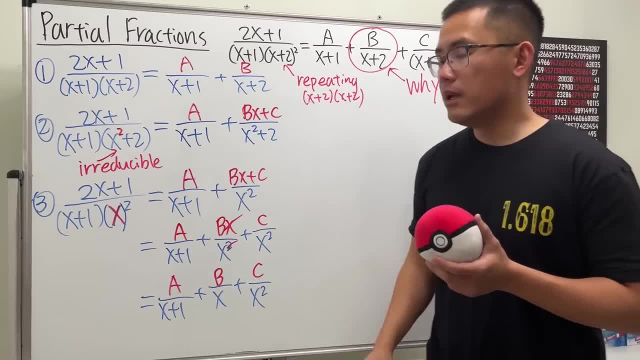 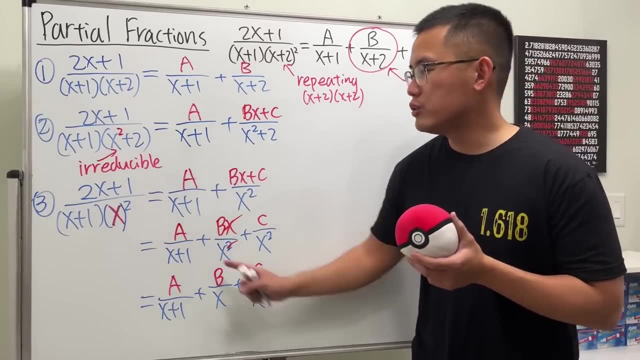 I call this build up the power. What it means is that you start with x to the first power, and then you build up, just keep adding 1 until you reach this power. 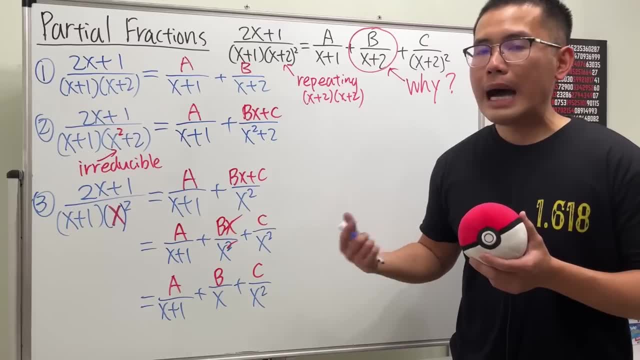 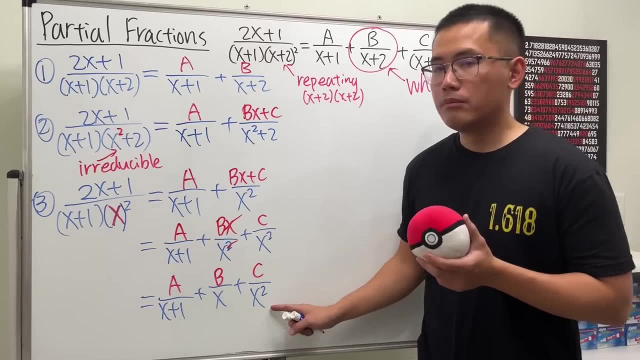 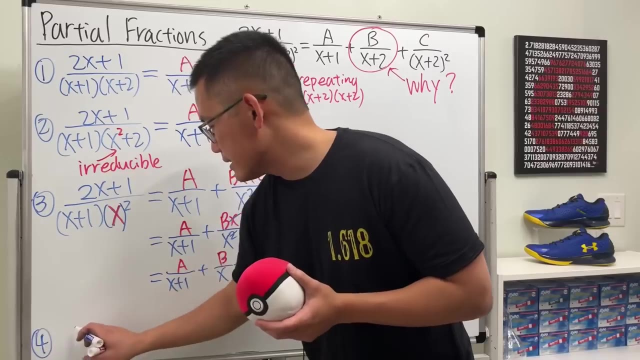 the first power. here I call this build up the power. What it means is that you start with x to the first power and then you build up, just keep adding 1 until you reach this power. Imagine if you have, let's say, let's say we have 2x plus 1 over, still x plus 1, but 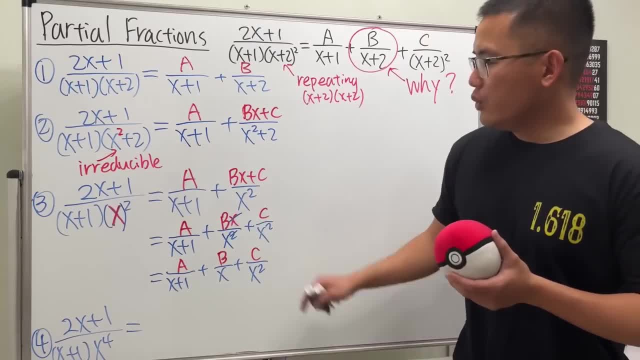 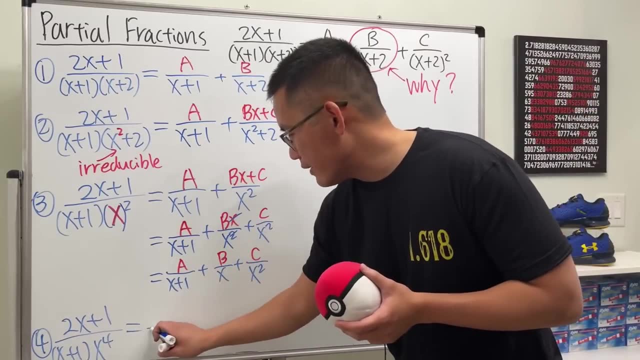 let's say we have x to the first power. Okay, You don't need to do this step every single time, Just remember: build up the power and set it up correctly. Firstly we will have x plus 1, and then the top will be a constant. let's say a. 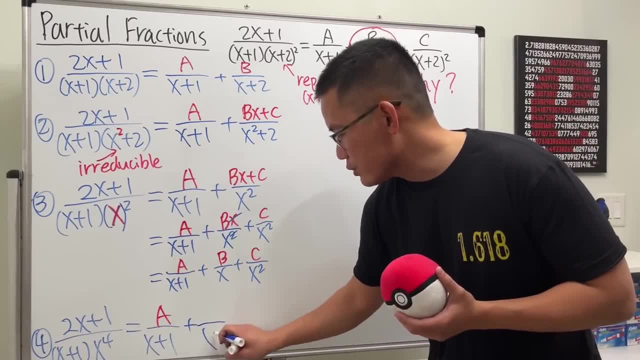 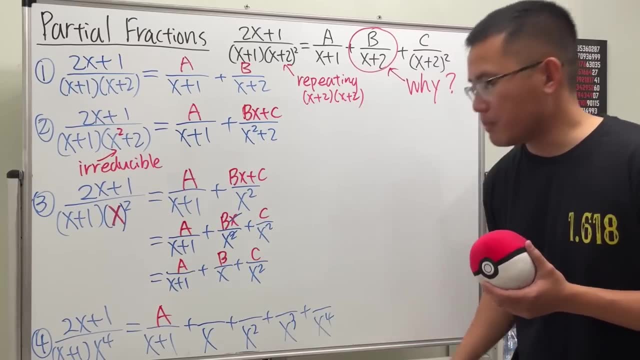 Okay, x to the fourth power. so here we go: Start with x to the first power, and then we just keep going: x squared, and then x plus third power, and then x to the fourth power. This right here is linear, so that means the top will be a constant b. 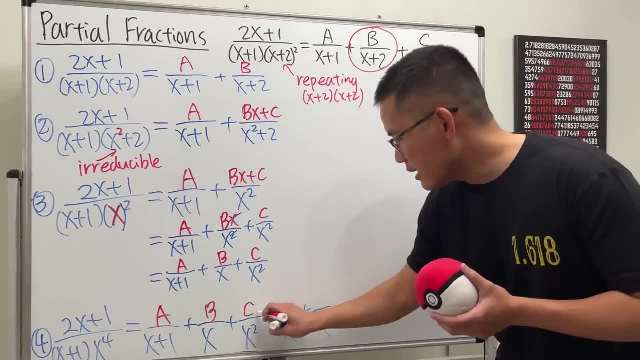 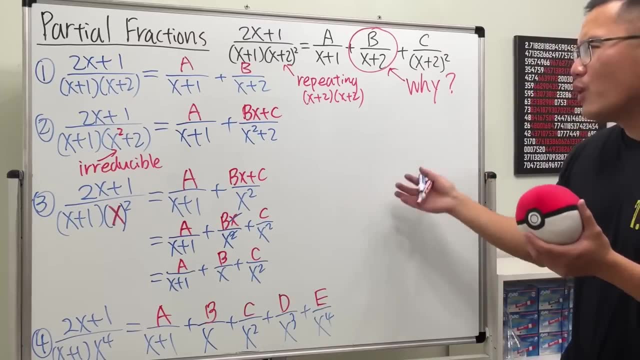 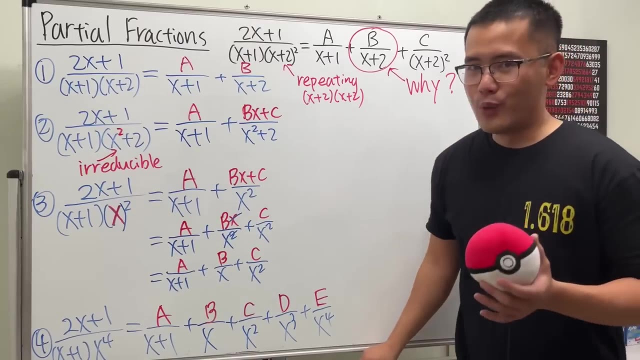 And then the top will stay the same time. So another constant, another constant, another constant. all right, So that's why we do that. but of course you would be thinking that this is x squared. this is just x. it might be different. 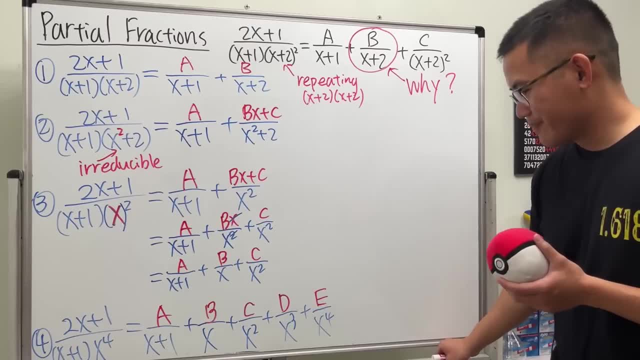 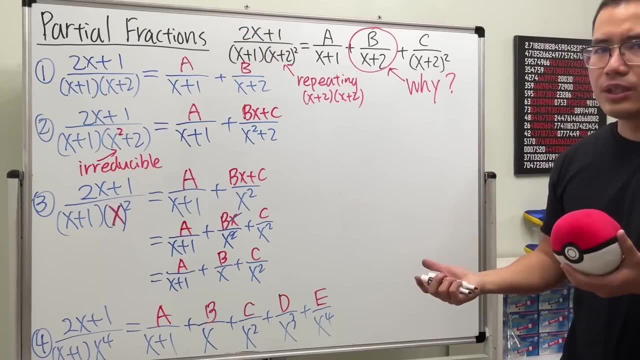 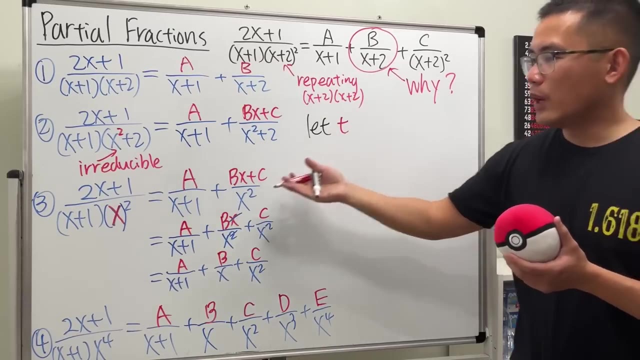 Don't worry, I got you. This is how you can explain this right here. So have a look. We still want to answer this expression. What we can do is just do some substitution And let's just say that, And I will just say that t equal to this, so that we will end up with a similar form. 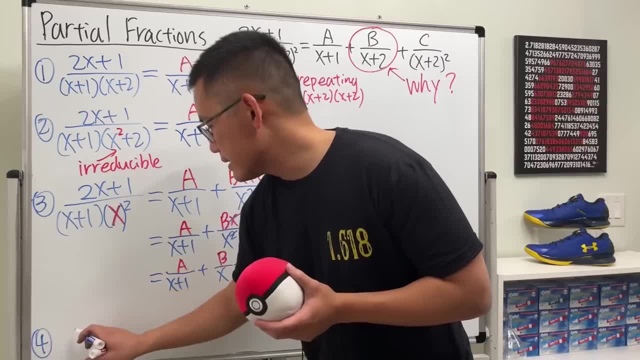 Imagine if you have, let's say, let's say we have 2x plus 1 over still x plus 1, but let's say we have x to the first power. Okay. 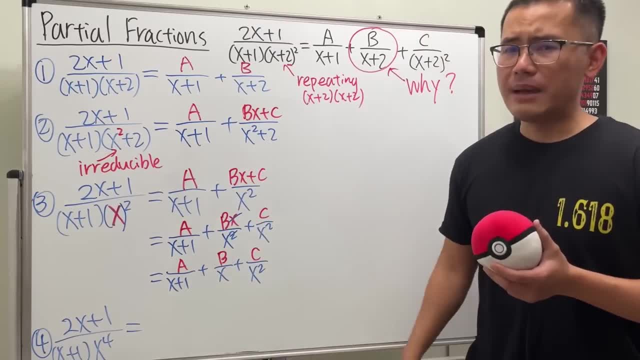 You don't need to do this step every single time. Just remember, build up the power and set it up correctly. 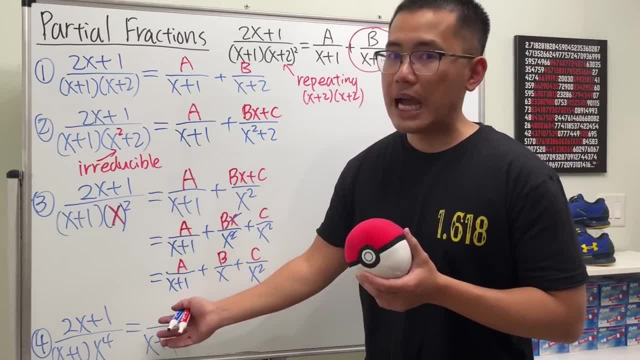 Firstly we will have x plus 1, and then the top will be a constant, let's say a. Okay. 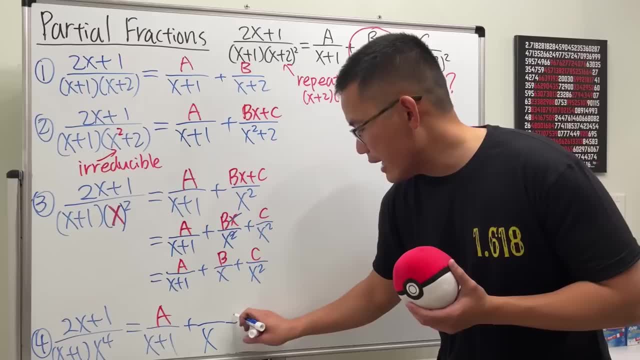 x to the fourth power. So here we go. Start with x to the first power, and then we just keep going, x squared, and then x 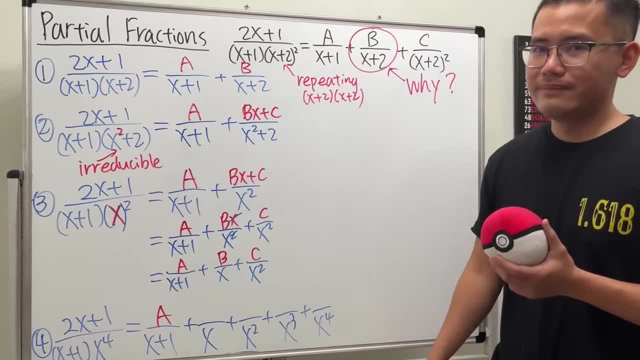 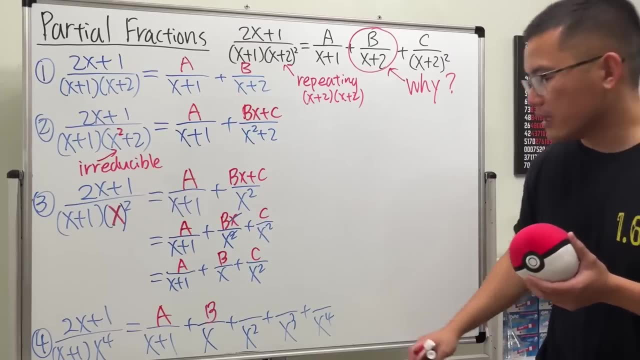 plus third power, and then x to the fourth power. This right here is linear. So that means the top will be a constant. B. And then the top will stay the same time. 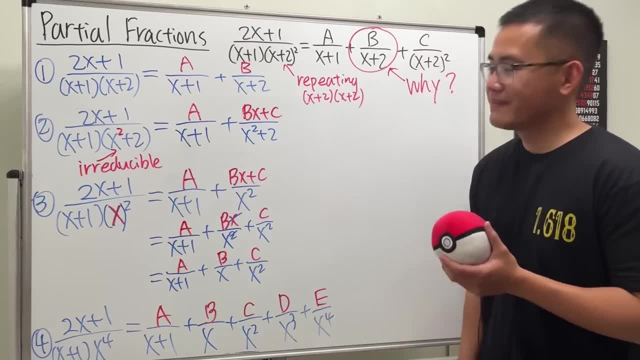 So another constant, another constant, another constant. All right. So that's why we do that. 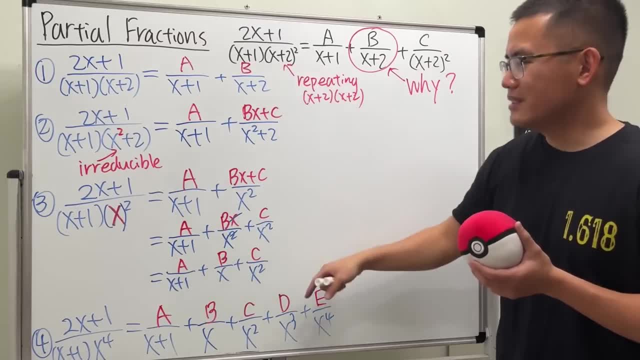 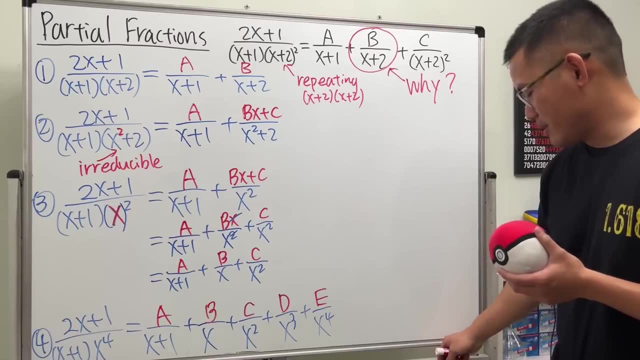 But of course you would be thinking that this is x squared. This is just x. It might be different. Don't worry. I got you. This is how you can explain this right here. So have a look. 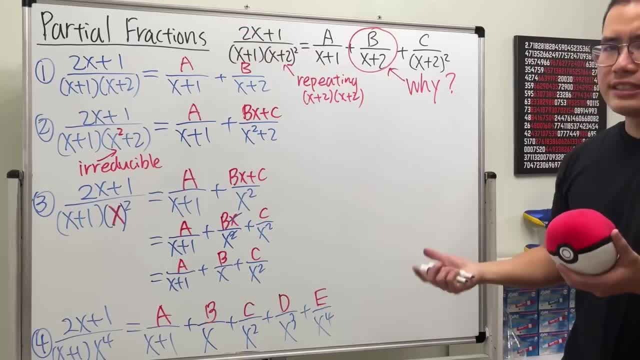 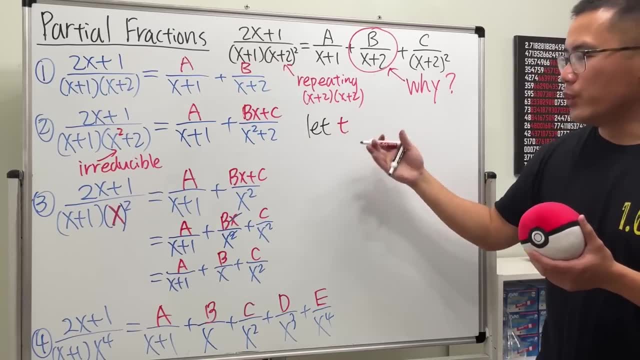 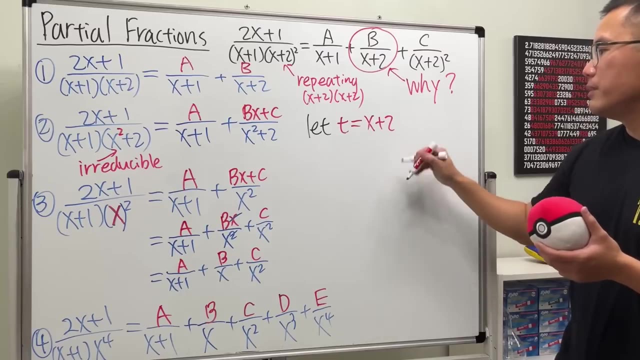 We still want to answer this expression. What we can do is just do some substitution. And let's just say. Let's say that t. And I will just say that t equal to this. So that we will end up with a similar form. So I'll just say t equals x plus two. And then we can do a few things, right? Because for example, we can say this is the same as saying x is equal to t minus two. 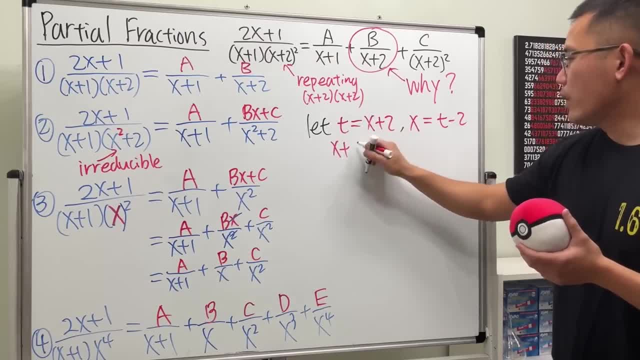 And then we can say x plus one. Just add one on both sides. 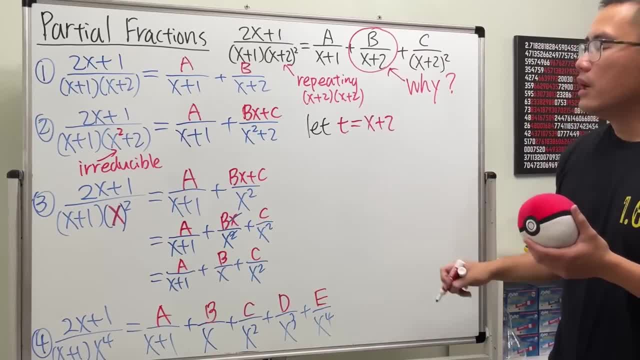 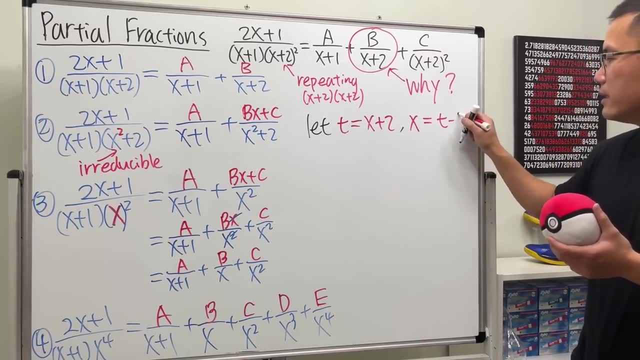 So I'll just say: t equals x plus 2.. And then we can do a few things right, Because for example, we can say: this is the same thing: x is equal to t minus 2.. And then we can say: x plus 1, just add 1 on both sides. 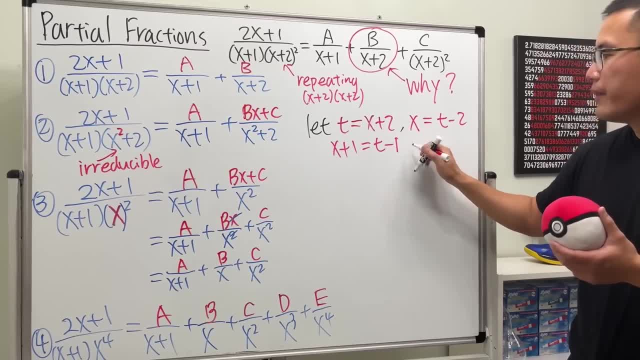 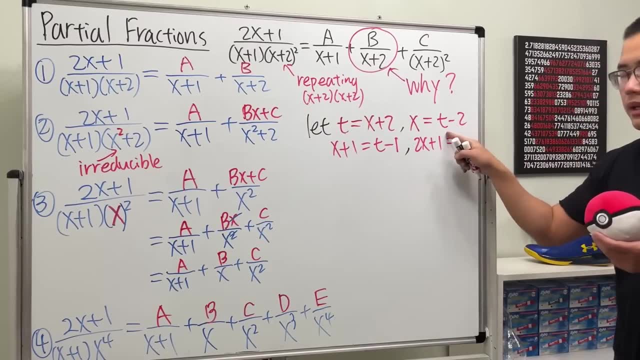 So x plus 1 will be t minus 1.. And then we also need a top which is 2x, And then we also need a top which is 2x plus 1.. Okay, let's do this in our head. 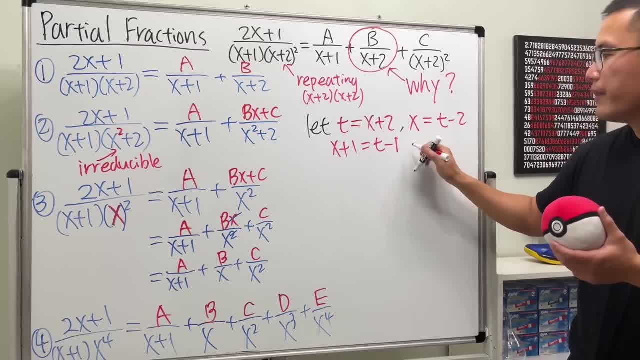 So x plus one will be t minus one. And then we also need a top, which is two x. Plus one. Okay. 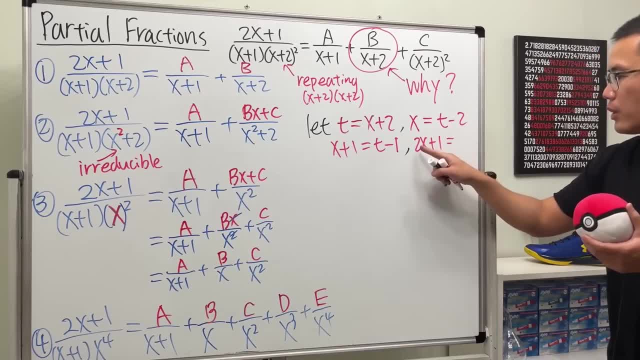 Let's do this in our head. So this will be two times t, which is two t. And then two times minus two is minus four. And then plus one is minus three. Okay. 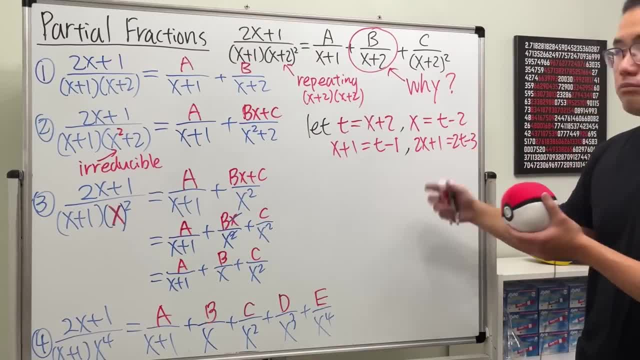 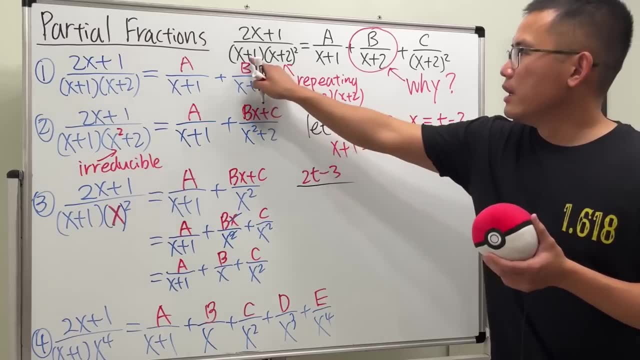 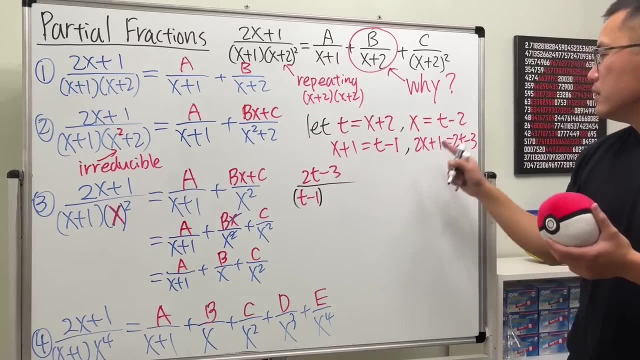 So we can look at this expression as what? The top is two t minus three. So let's write that down. And then over x plus one is that. T minus one. And then the x plus two is t. So we have the t squared. 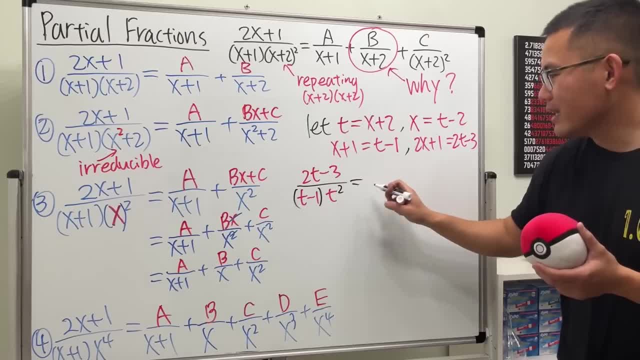 And now per our discussion earlier, this right here will just be what? 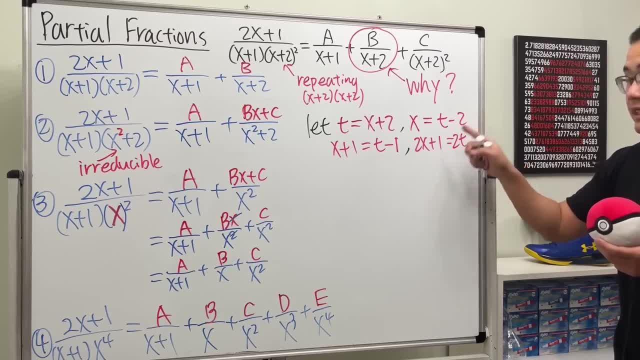 So this will be 2 times t, which is 2t, And then 2 times minus 2 is minus 4.. And then plus 1 is minus 3.. Okay, so we can look at this expression as what The top is: 2t minus 3.. 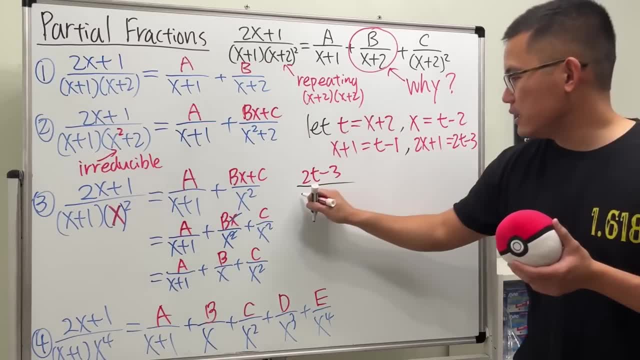 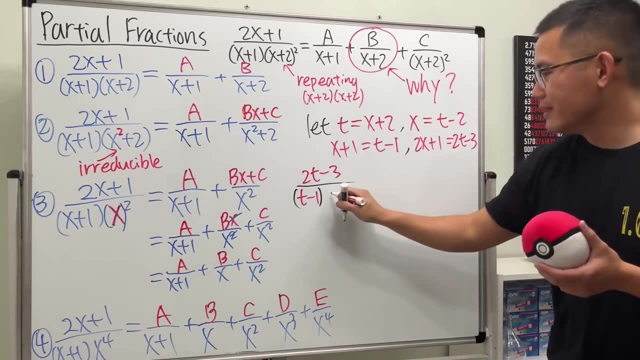 So let's write that down, And then, over x plus 1 is that t minus 1.. And then the x plus 2 is t, So we have the t squared. And now, per our discussion earlier, this right here will just be what. 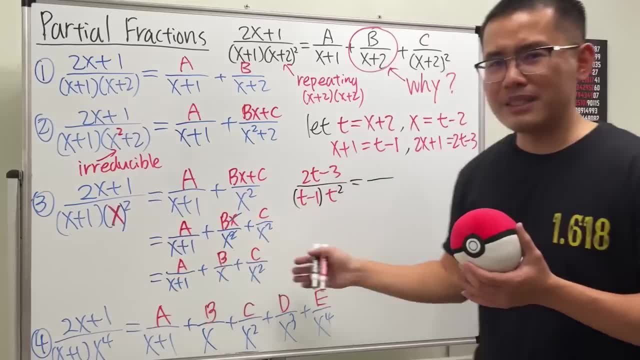 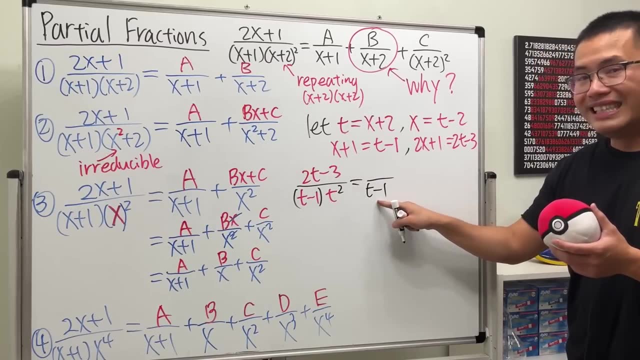 t minus 1, even though we have the plus 1.. But again, it's the form, It's not about the number. This right here is t minus 1.. It's linear. The top will be a constant And likewise this right here will be okay. build up the power. 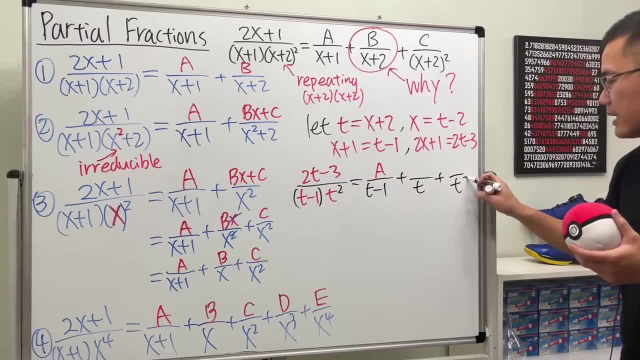 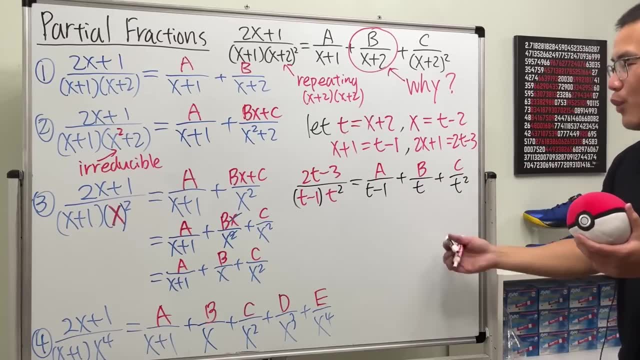 t to the first And then t to the second. The top will just be a constant. Likewise, the top will be a constant. We're all done, huh? And of course, in the end we can set this back just to match it. 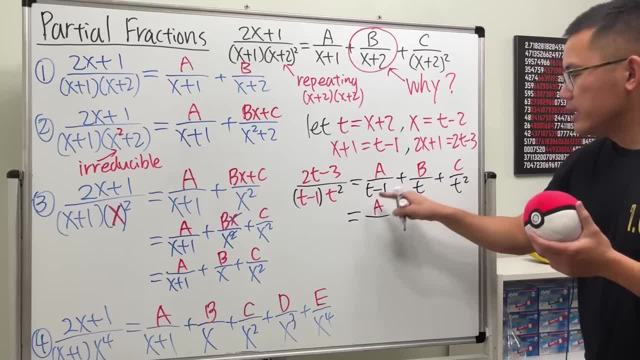 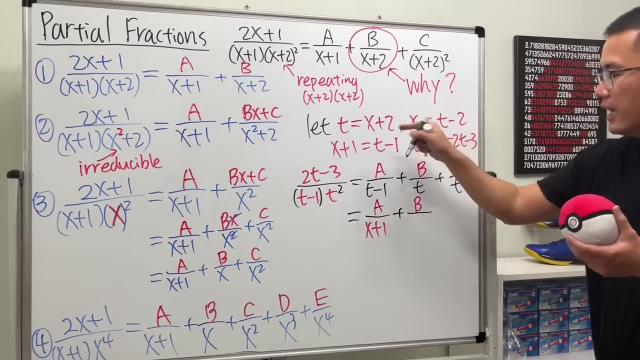 So, ladies and gentlemen, a over t minus 1 is x plus 1.. So we can put that down, And then b, And then t is x plus 2.. And of course, lastly, we have that c over x plus 2.. 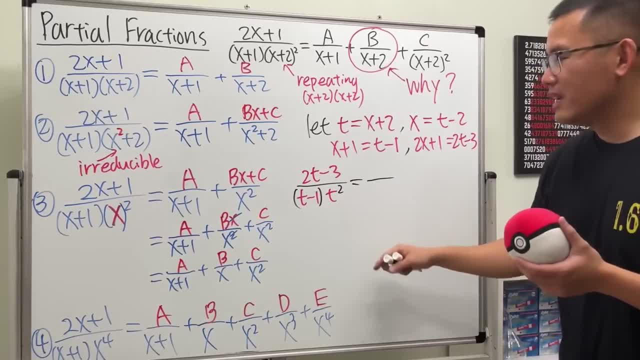 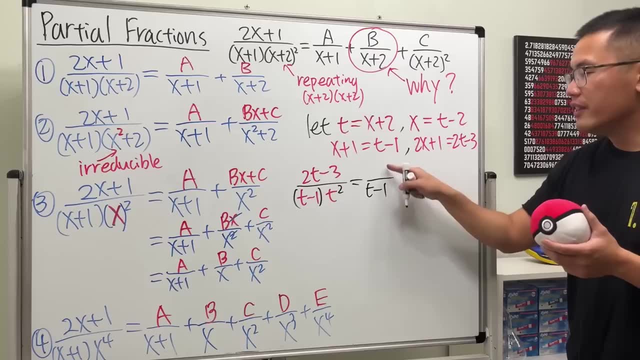 T minus one, even though we have the plus one. But again, it's the form. It's not about the number. This right here is t minus one. It's linear. The top will be a constant. And likewise, this right here will be, okay, build up the power. T to the first. 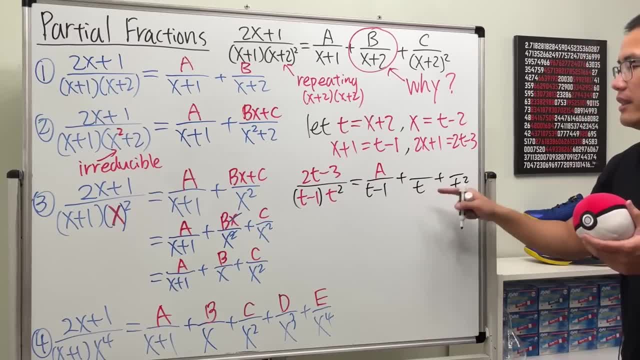 And then t to the second. The top will just be a constant. Likewise, the top will be a constant. We're all done, huh? 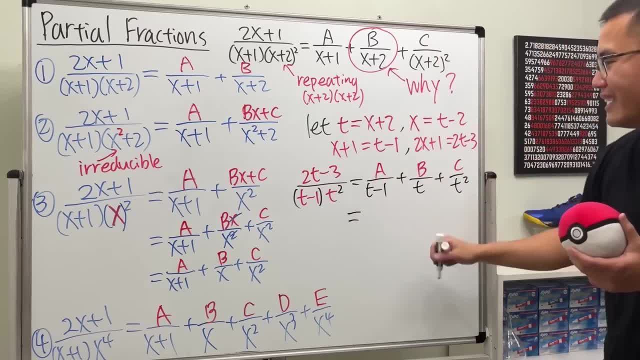 And of course, in the end, we can set this back just to match it. So ladies and gentlemen, a over t minus one is x plus one. 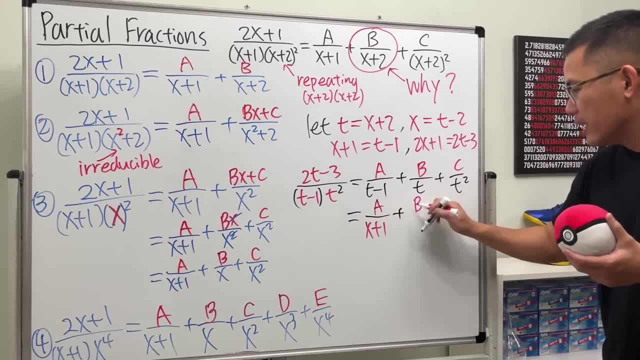 So we can put that down. And then b. And then t is x plus two. 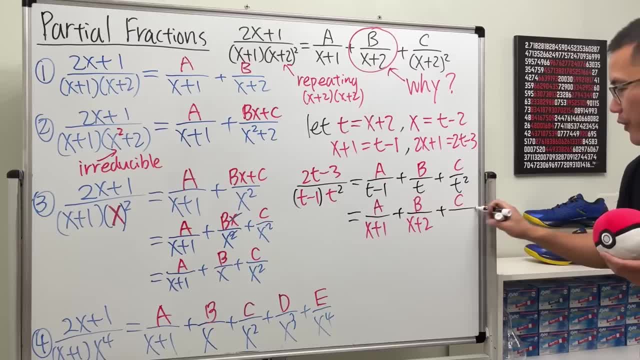 And of course, lastly, we have that c over x plus two. Okay. So we can put that down. And then square. 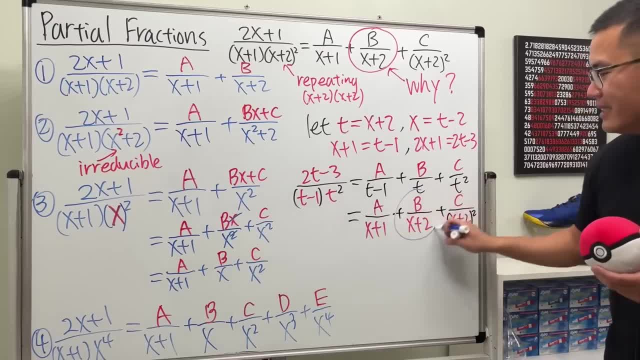 So ladies and gentlemen, this is the reason why that we must have this term right here. Hopefully, this video helps. 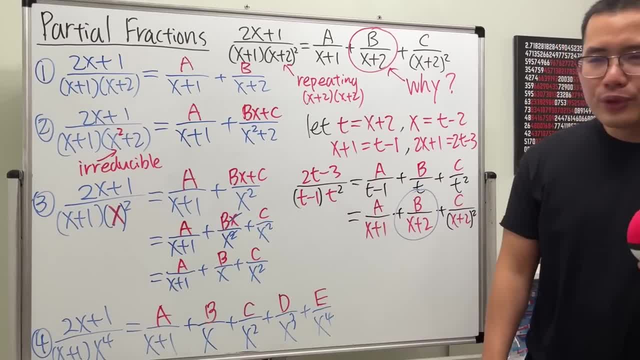 For more tutorials, for more tutorials, for more tutorials. 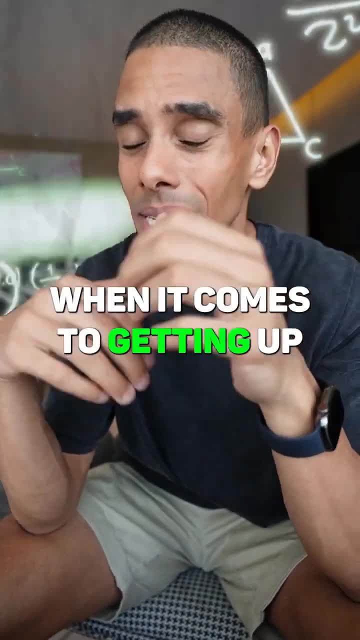 Linear algebra is one of the foundation concepts when it comes to getting up to speed with machine learning. But did you know that NumPy can help streamline a bunch of this for you? Let's take 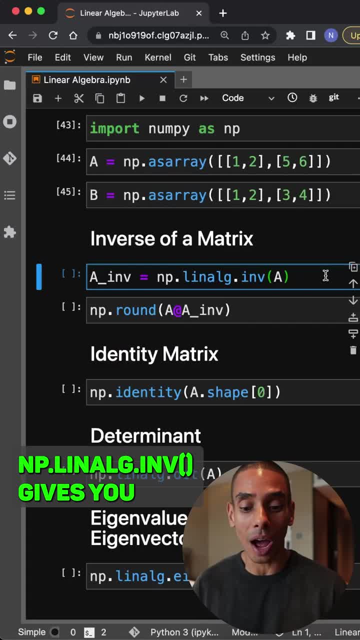 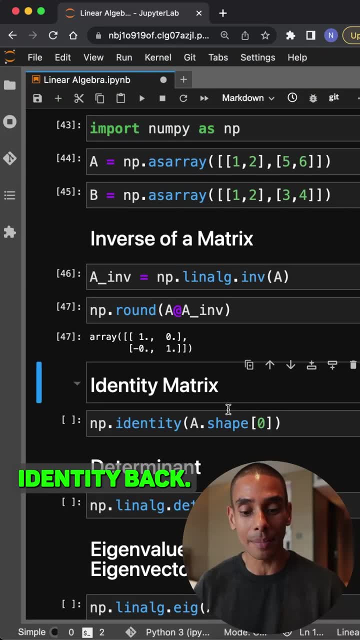 a look at some of the shortcuts that NumPy gives you. np.linalg.inv gives you the inverse of a matrix. In this particular case, if we multiply the original matrix by the inverse, you can see we're getting the identity back. If we want to get the identity matrix, we can use numpy.identity 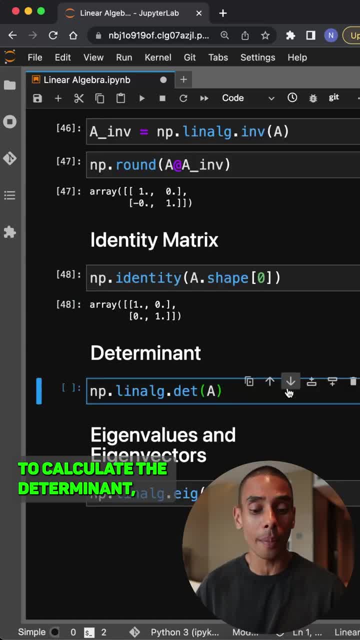 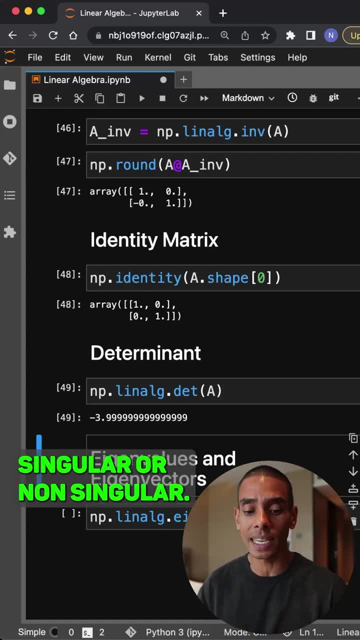 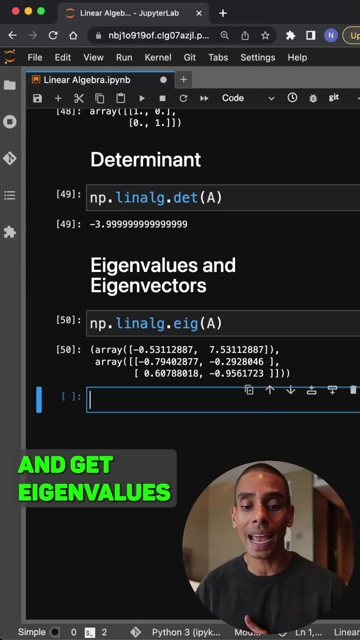 and pass through the shape of our original matrix. To calculate the determinant, we can use numpy.linalg.det and this will give us the determinant of our matrix telling us whether or not it's singular or non-singular. And last but not least, eigenvalues and eigenvectors. By using numpy.linalg.ig, we're able to go on ahead and get our eigenvalues and our eigenvectors. 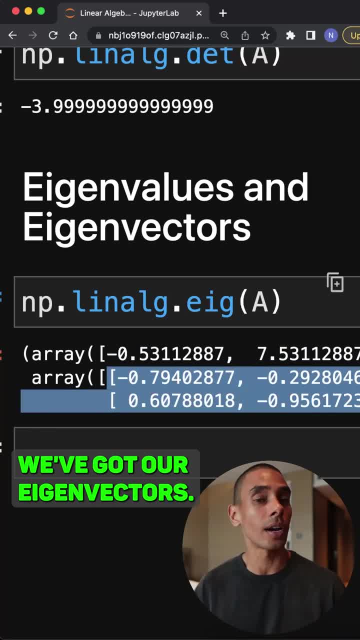 At the top, you can see we've got our eigenvalues and down the bottom, we've got our eigenvectors. Work's already begun on my math for ML course. You pumped for it?